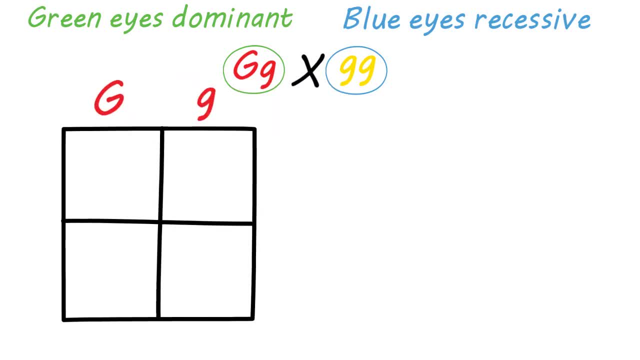 square. One of the parental genotypes will go on top and the other will go on the side. It doesn't matter which genotype goes where. It doesn't matter which genotype goes where, It doesn't matter where, and the order of the letters really doesn't matter. But we conventionally write: 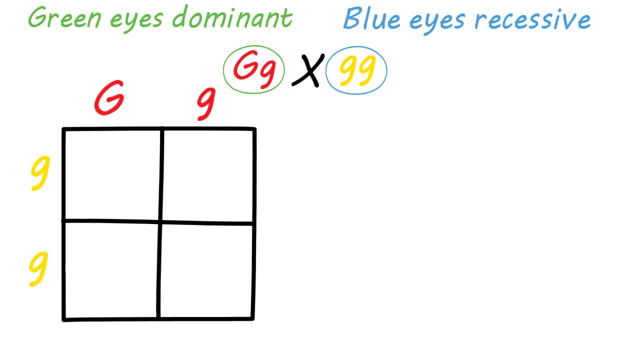 the dominant allele first. if there is a dominant allele, So your setup should look like this. Then you simply carry the letters through to their respective quadrants and match them up like. so Each quadrant will represent a 25% chance that that genotype will result in the offspring. 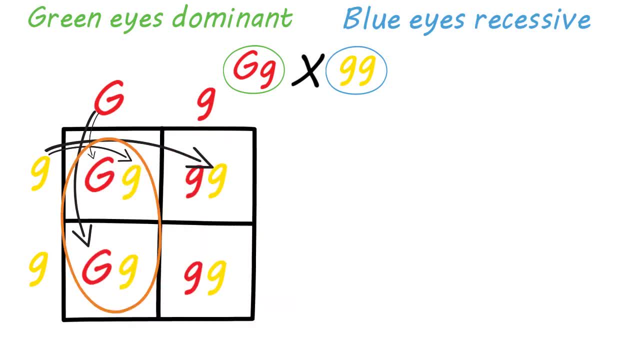 So in this case we have only two possible genotypes- big G, little g and little g- little g- And each genotype has a 50% chance of showing up in the offspring. So in this case we have only two possible genotypes- big G, little g and little g- little g- And each genotype has a 50% chance of showing up in the offspring. 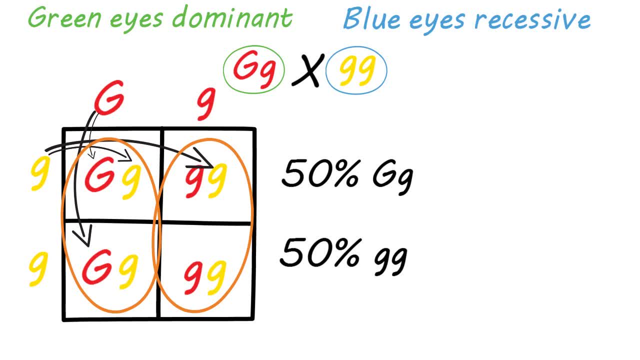 Similarly, you have two possible phenotypes- green eyes and blue eyes, with a 50% chance of each. Let's look at another example. We'll cross two genes that are heterozygous for eye color in this example. So Big G, little g crossed. 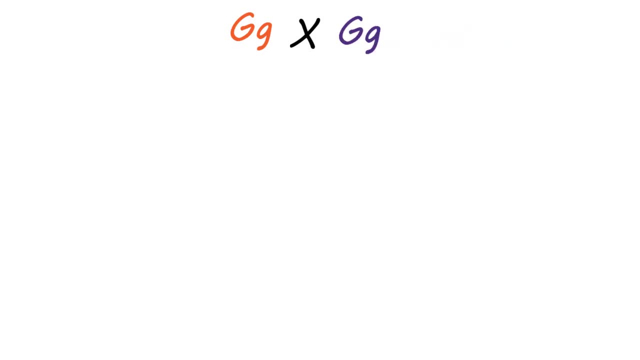 with Big G, little g. These colors are just for illustration purposes. So we again, we'll draw up Punnett square and put one gene on top and the other down the side, Then carry letters through to their respective quadrants and analyze their results. 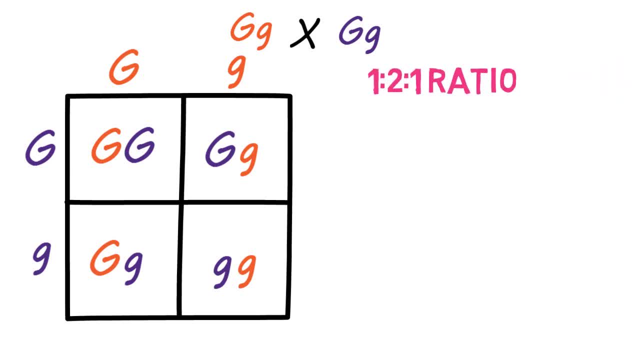 So this cross results in a 1 to 2 to 1 genotype ratio with 25% homozygous dominant or big G, big G, 50% heterozygous or big G, little G, and 25% homozygous recessive or little G, little G. 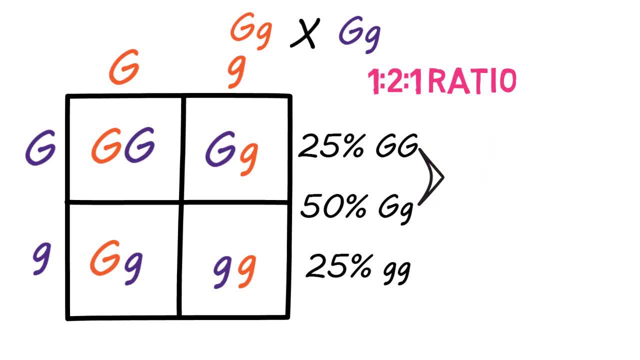 The phenotypic ratio would be a 3 to 1 ratio, with 75% green eyes and 25% blue eyes. Hopefully that helps you understand simple Punnett squares a little better. Genetic crosses can be much more complicated and I'll make a video sometime in the future. 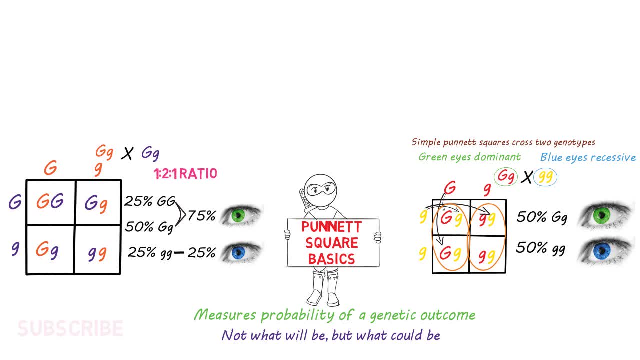 explaining how to tackle those more complicated genetic crosses. If you have any questions from this video, throw them in the comments, and don't forget to like and subscribe. Thanks for watching. I'll catch you next time.